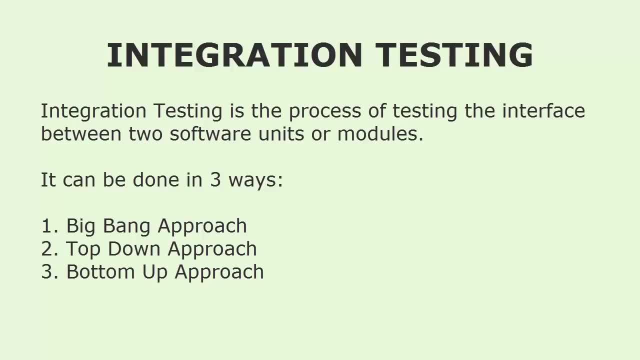 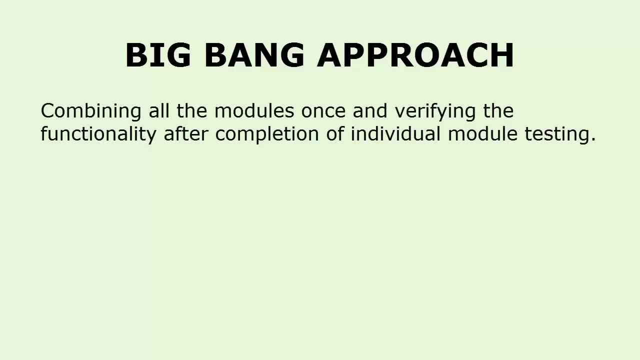 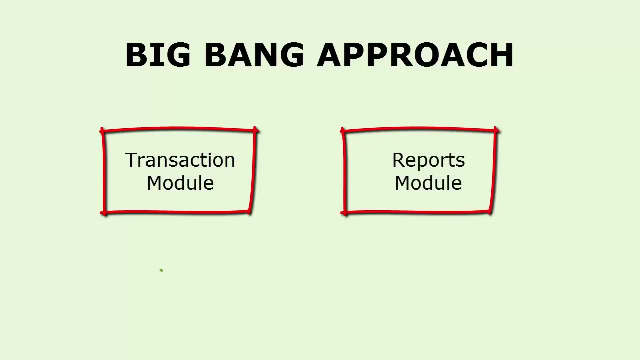 top-down approach and bottom-up approach. So what is Big Bang approach? Combining all the modules once and verifying the functionality after completion of individual module testing. Assume we have two modules, such as transaction module and reports module. First we do testing. 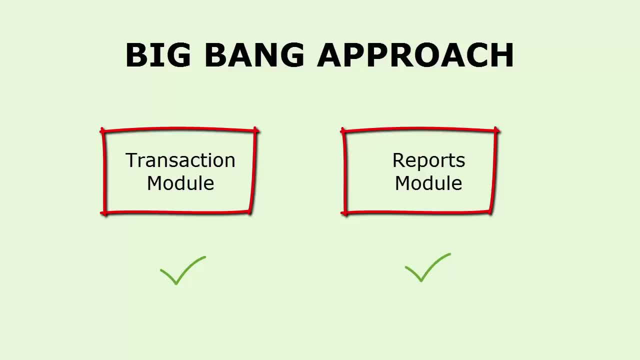 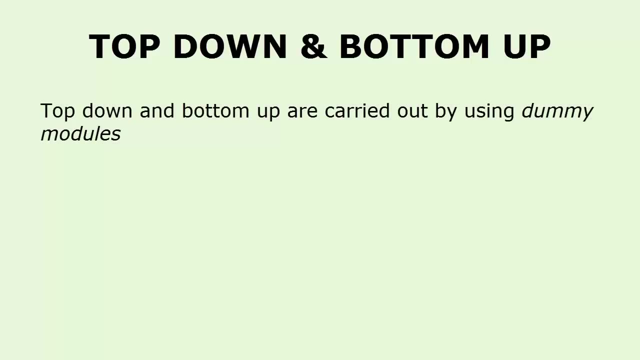 on both the modules individually And then we do testing on both the modules after combining the two modules. What is top-down and bottom-up approach? Top-down and bottom-up are carried out by using dummy modules known as stubs and drivers. These stubs and drivers are used to stand. 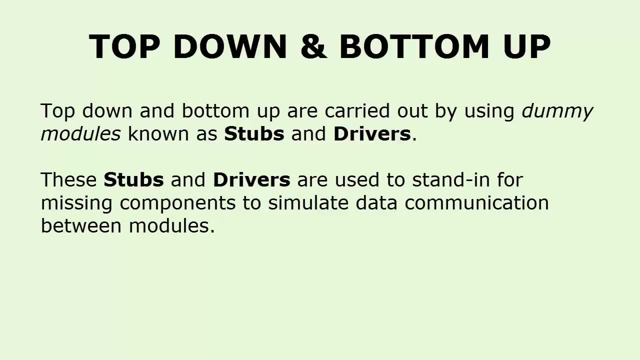 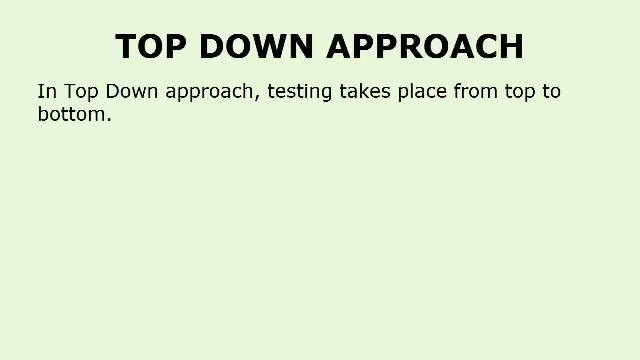 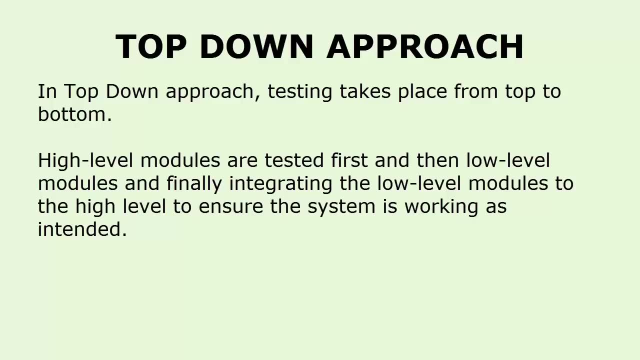 in for missing components. to stimulate data communication between modules In top-down approach, testing takes place from top to bottom: High level modules are tested first and then low level modules and finally integrating the low level modules to the high level to ensure the system is working as intended. 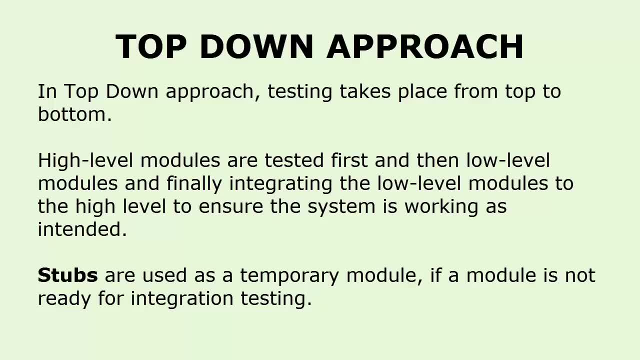 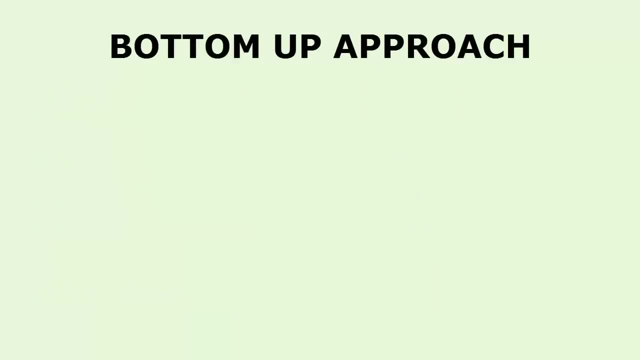 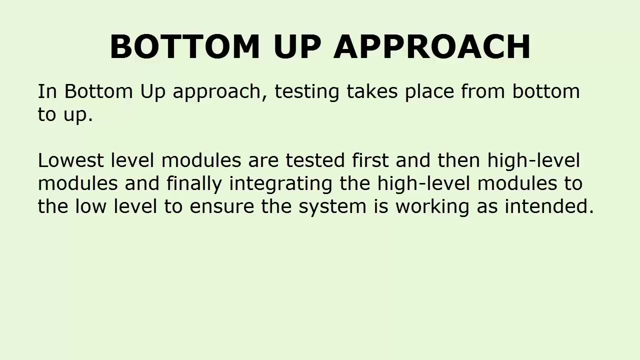 Stubs are used as a temporary module if a module is not ready for integration testing. Moving to bottom-up approach: Bottom-up approach is a reciprocate of the top-down approach. Testing takes place from bottom to up: Lowest level modules are tested first, and then high level modules and finally integrating. 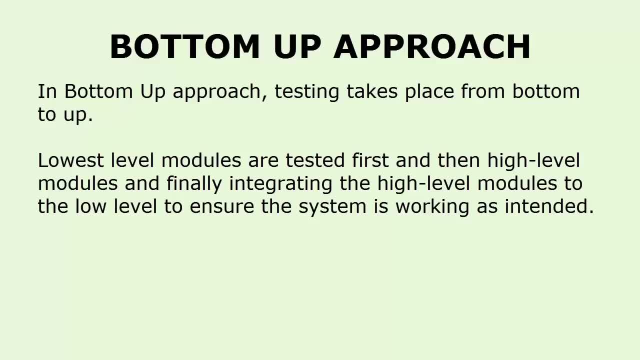 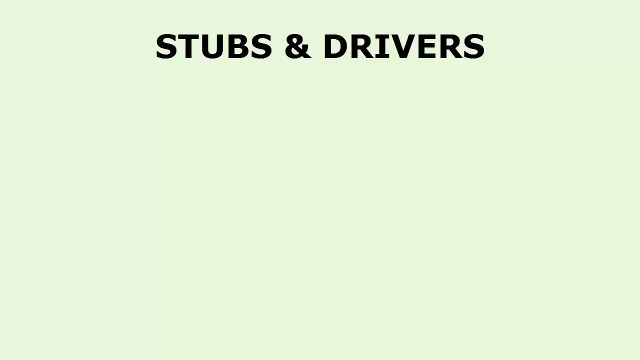 the high level modules to the low level to ensure the system is working as intended. Drivers are used as a temporary module for integration testing. Let's move to bottom-up approach. Let's see Drivers and Stubs in detail. These terms come into the picture while doing integration testing. 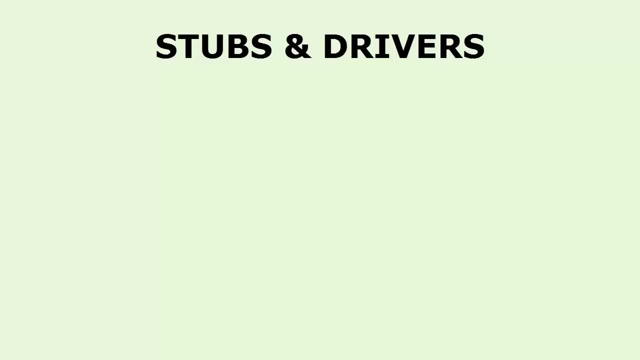 While working on integration, sometimes we face a situation where some of the functionalities are still under development, So the functionalities which are under development will be replaced with some dummy programs. These dummy programs are named as Stubs or Drivers. Assume we have two pages, login page and admin page.